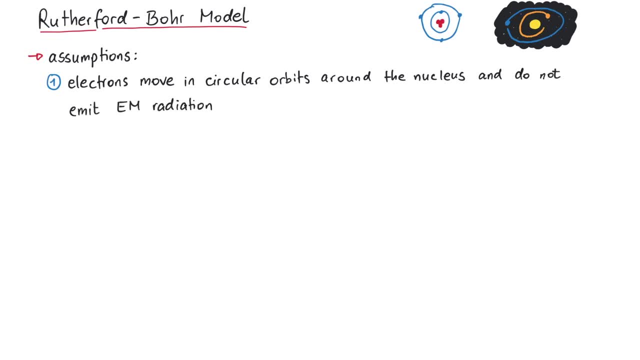 electromagnetic radiation, even though, according to classical electromagnetism, an accelerated charge should emit this kind of radiation. Such orbits are also called stationary orbits. Second, these stationary orbits have discrete radii, so it's not possible to be in between two orbits. This can be expressed mathematically via: the Rutherford-Bohr model. The Rutherford-Bohr model is based on the Rutherford-Bohm model. The Rutherford-Bohm model is based on the Rutherford-Bohm model. The Rutherford-Bohm model is based on the. 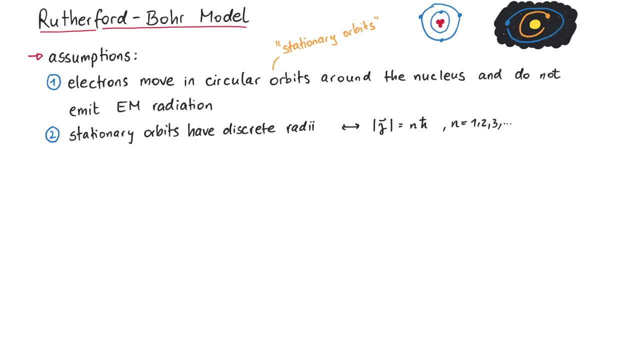 angular momentum of the electron, which must be an integer multiple of h-bar. Third, the electrons are allowed to jump from one orbit to another by receiving or emitting energy. The exact amount of energy depends on the energy difference between those two orbits. Now let's go into some more detail and assume that we're dealing with a one-electron system. 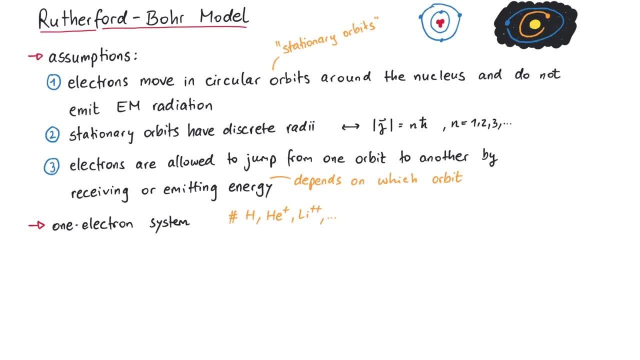 This could be a hydrogen atom, ionized helium or lithium atoms, and so on. as long as we don't have any electron-electron interactions, The electron on its circular orbit is bound to the nucleus via the Coulomb force, such that the centripetal force and the Coulomb force balance each other. 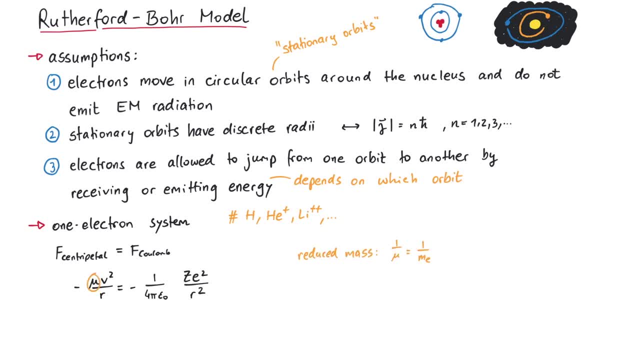 In this equation, mu stands for the reduced mass of the electron-nucleon system and z tells us how many protons are in the nucleus. since this determines how strong the nucleus pulls the electron towards it, We can rearrange this equation to give us the radius of the electron orbit, the. 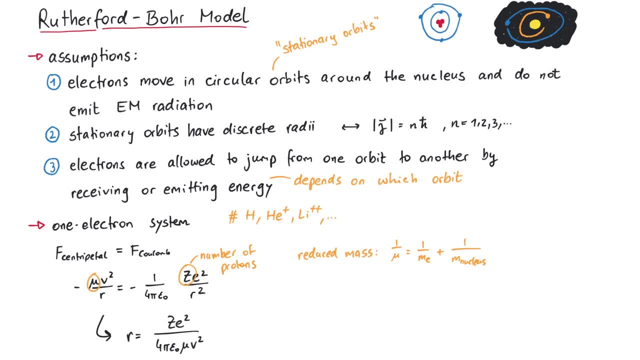 depending on its velocity. At this point we must make sure that there are only discrete orbits, as mentioned in the second assumption. By claiming that the angular momentum must be an integer multiple of h-bar, we can express the velocity of the electron in terms of this integer n. There's actually another equivalent way to get to this expression. 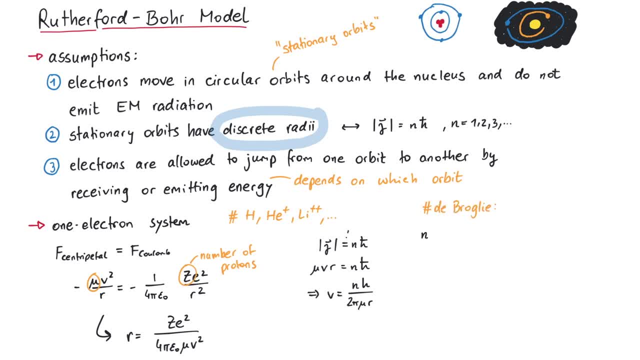 We can claim that the de Broglie wavelength of the electron must be able to fit n times within the circumference of the orbit. In other words, if we draw the wave along a circular orbit, we want the beginning and end to meet at the same point, resulting in a standing wave. Otherwise, 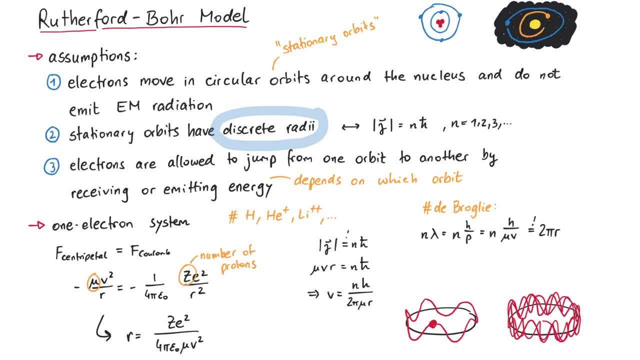 this would result in a cancellation of the wave due to destructive interference And really this yields the same relation for the velocity. Using this, we can express the radius in terms of n, z and some constants, which together are called A0, Bohr's radius.